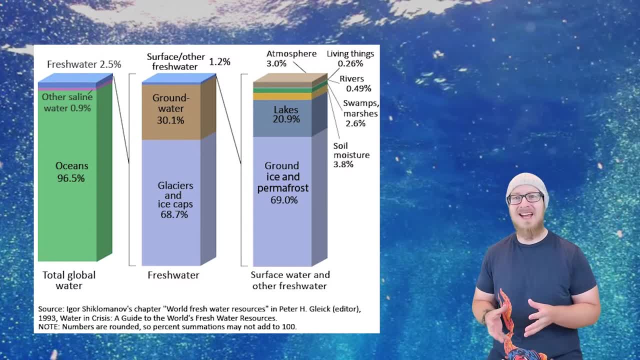 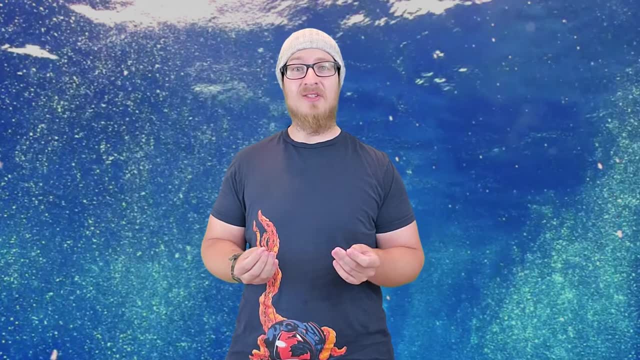 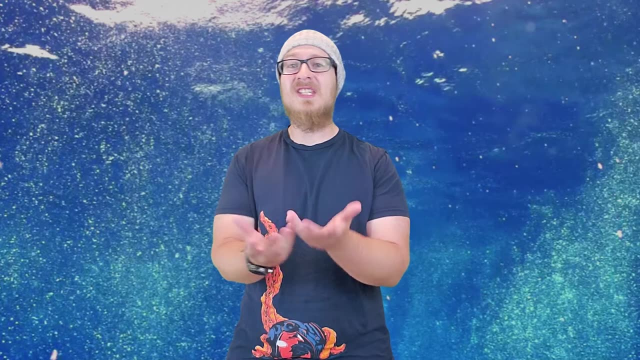 surface water is difficult because the majority of that is locked away in permafrost, frozen in soils. Usable water in the world is scarce, so how we use it matters, And the conservation of it is becoming of a growing importance. especially with the increasing population is increasing the 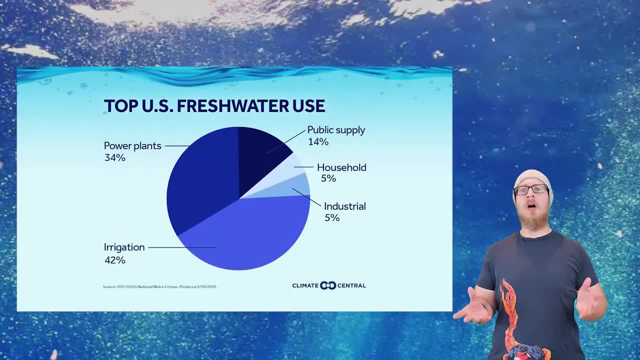 demand for clean water. The majority of water use comes from agriculture: for watering our crops and for livestock. The next largest use is in power plants. The public supply refers to water that we may not be directly responsible for, like firefighting or street cleaning, or the water that we use in parks. 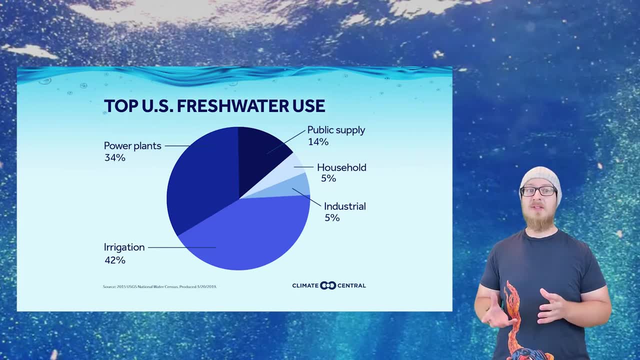 and swimming pools. The water use we are responsible for is the household use, which is our drinking water, and what we use for hygiene. Industrial water use is the water that is used for the processing, fabrication, cleaning and cooling of water. The water we use is stored in trucks and, at the end of the day, the water we use is the goods we purchase. 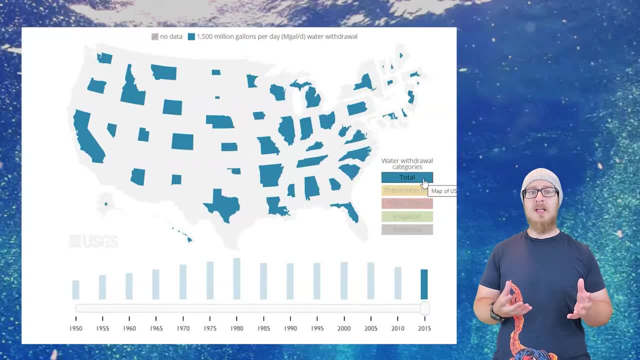 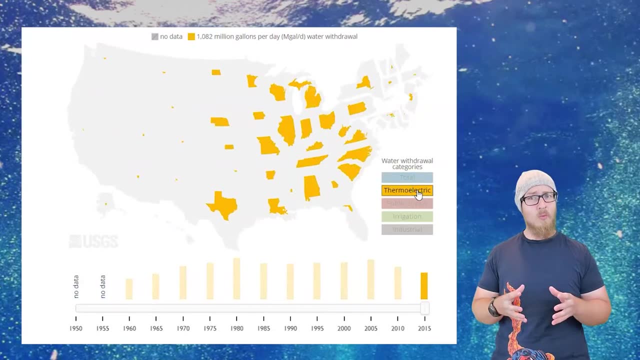 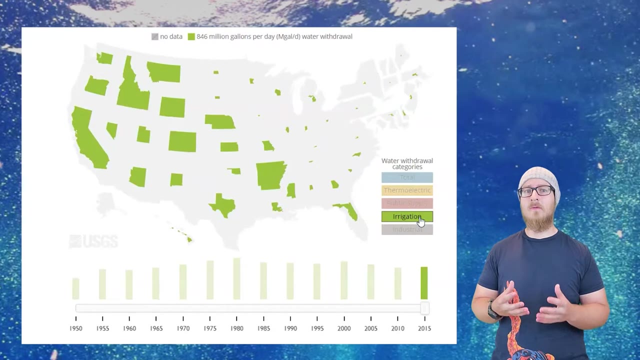 How that water is used is different in every state. Here we see the total water use in the United States scaled per state. The eastern half of the United States uses a lot of water for power generation, while the western half of the United States uses a majority of its water for the irrigation of crops. 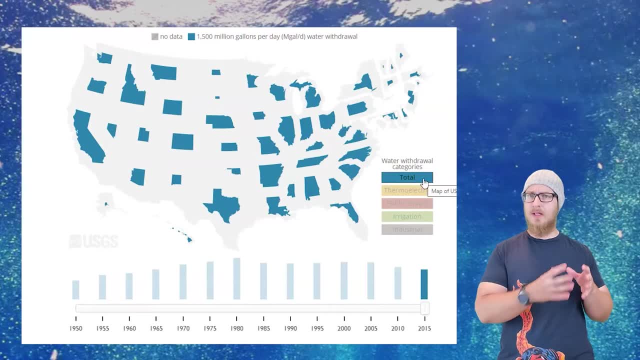 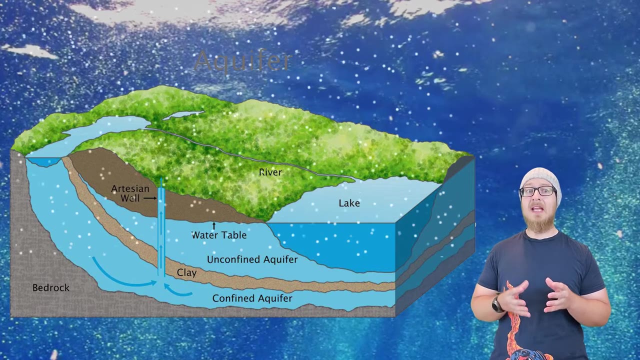 The majority of water used in the east comes from surface waters like lakes and rivers. United States and the central United States, the majority of it comes from groundwater. Now we get to this by building wells, but we have a concern with it. See, groundwater can be. 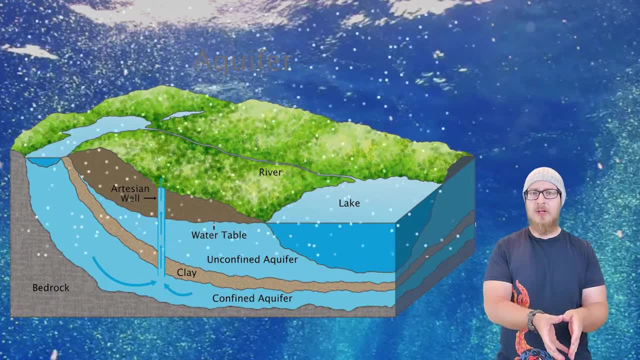 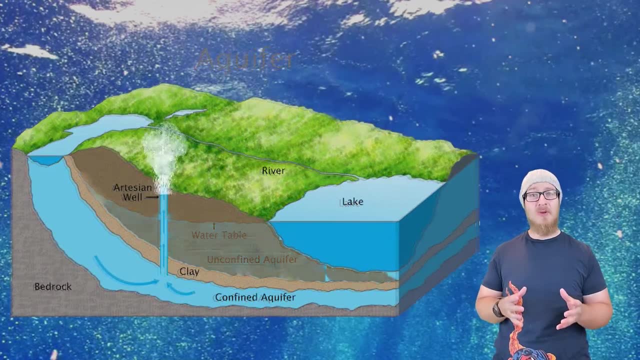 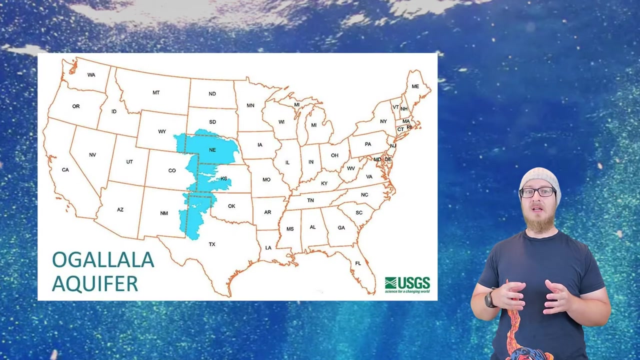 recharged as rain falls and infiltrates and percolates back into groundwater sources, but right now we're extracting water faster from the ground than it is being recharged For one that's unsustainable: The Agalala Aquifer, which provides the vast majority of water. 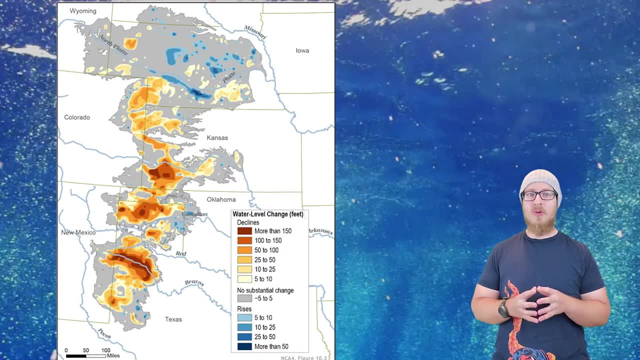 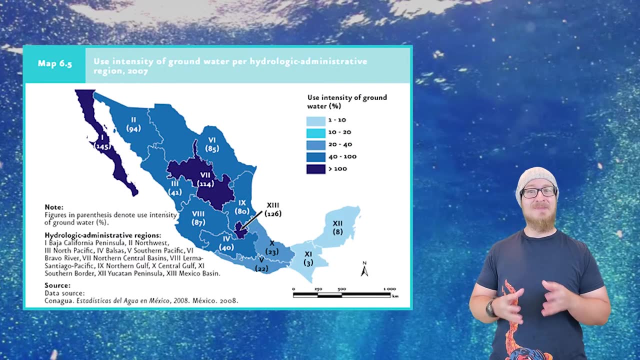 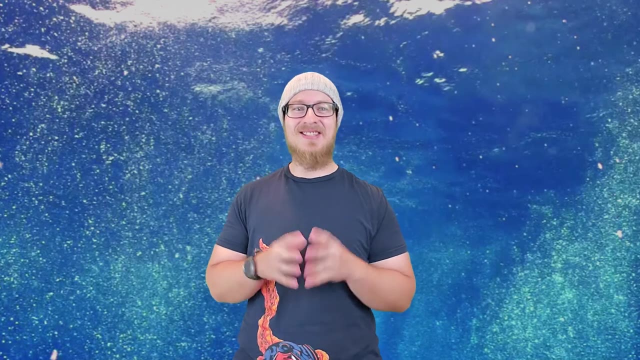 in the central United States has dropped by more than 150 feet worth of water in some places. The aquifers below Mexico City is being depleted so quickly that Mexico City is sinking. Now that animation is a little exaggerated, but we can visibly see. 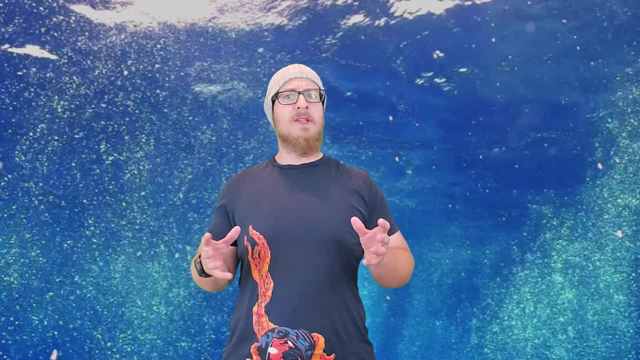 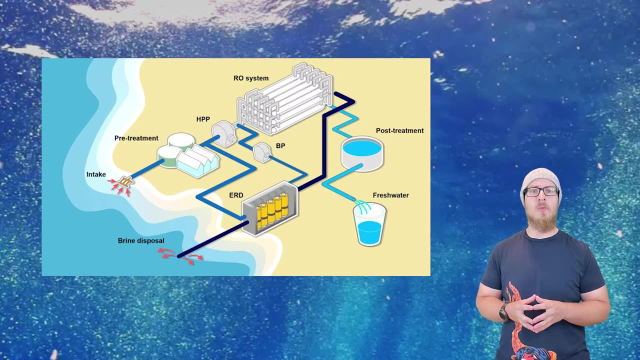 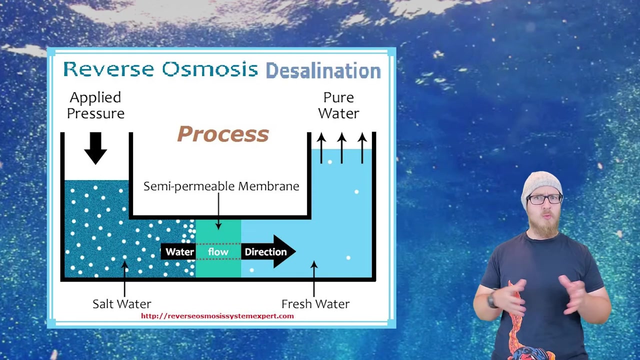 buildings sinking down. Now we do have some solutions to this water crisis. One method is to desalinate or remove the salt from ocean water to make it drinkable and usable for crops. This process involves using reverse osmosis, which pushes water through a membrane that is permeable to water but not to salt. Well, the issue here is that all that salt must be disposed of in some way, and most of the time it gets discharged back into the ocean. Even saltwater fish have a tolerance to salinity, and if it gets too high they may not be able to. 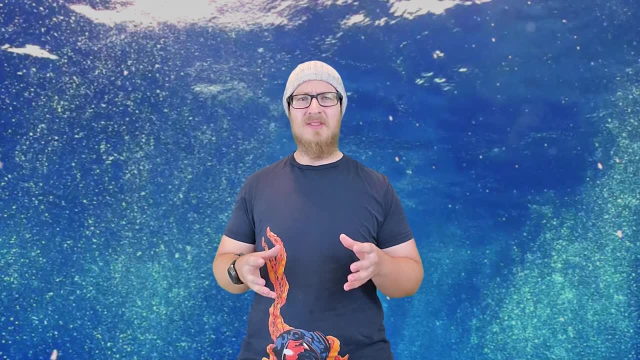 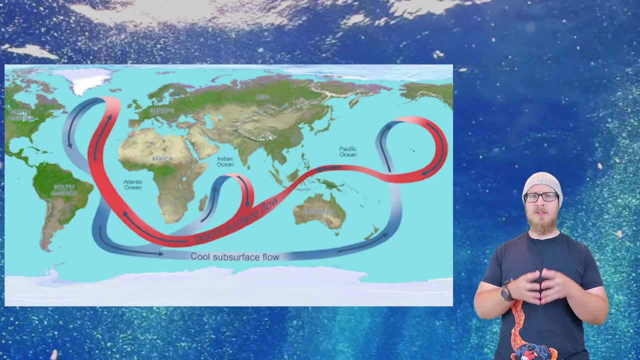 survive near the discharge area. Another point: the saltwater is denser, which makes it sink to the lower parts of the ocean. The global flow of ocean water, this circulation pattern we see on this map, are already changing as a result of ice melt from the Arctic due to global warming. 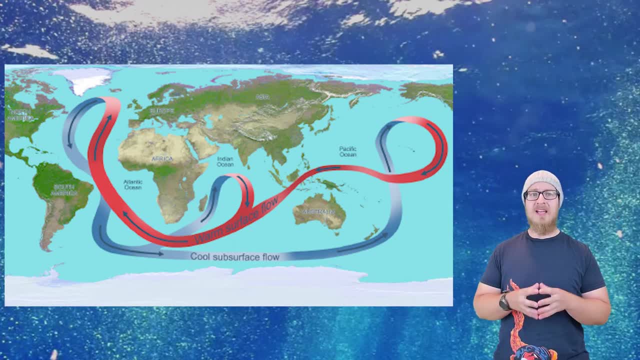 A change in the flow of this ocean water is a huge risk to the sea and the sea is a big risk to the water. can affect how storms form. it can affect the economy- I mean especially in places where fishing is a major industry- and alter the food webs in ocean ecosystems Right now: desalination. 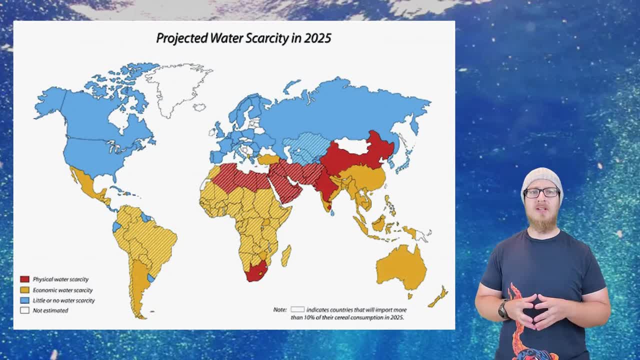 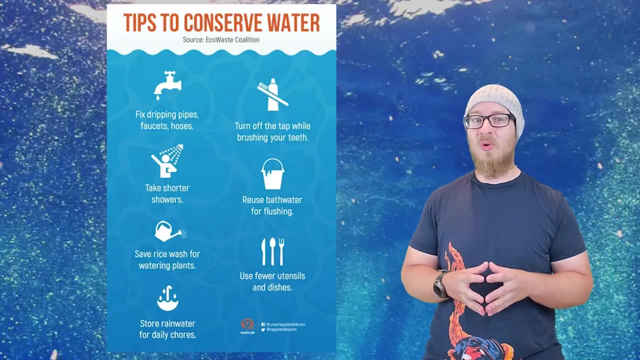 doesn't contribute greatly to the changing ocean circulations, but an increasing demand for water may increase the use of desalination and add to this change. At the end of the day, the best thing we can do is conserve the water resources we already have. Use less water at home by fixing. 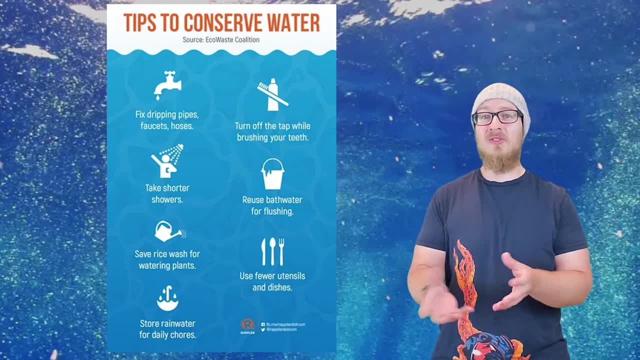 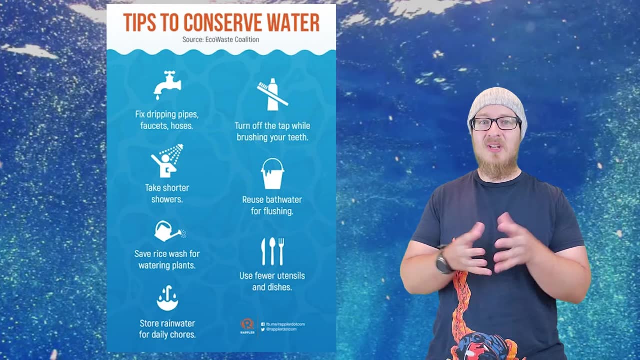 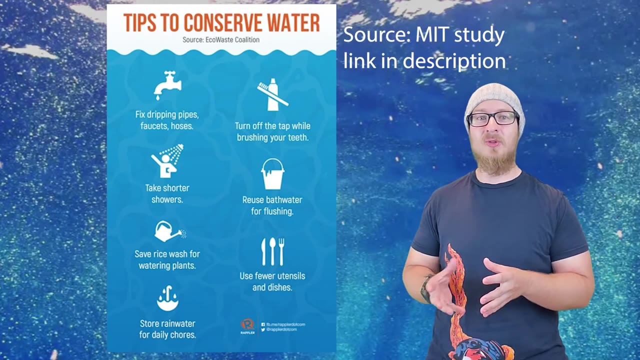 leaks, taking shorter showers and only using washers if you have a full load. While this seems small, by using water saving features like those, you can reduce your in-home water use by up to 35%. This means the average household, which uses about 13,000 gallons per year, could save 44,000. 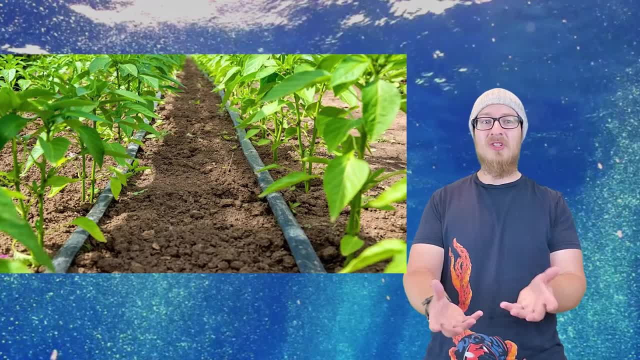 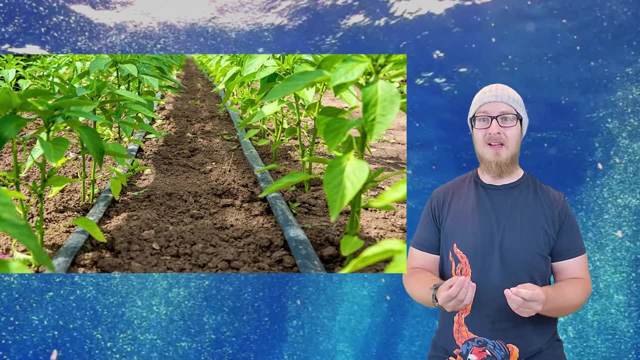 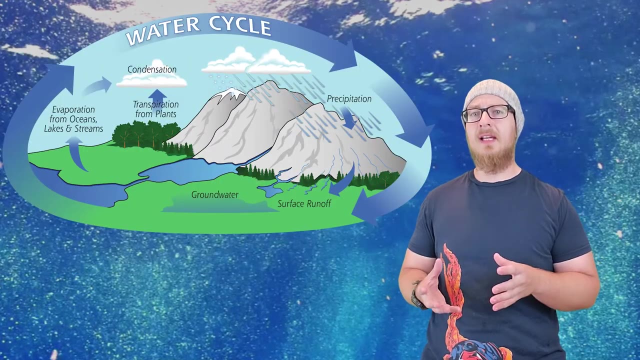 gallons of water. In agriculture, we can use more efficient watering systems like drip irrigation, which reduces a farm's water use by up to 60% And even more so, it can actually increase crop yields by 90%. All the water we use is inherently linked by the hydrological cycle that we covered before, but